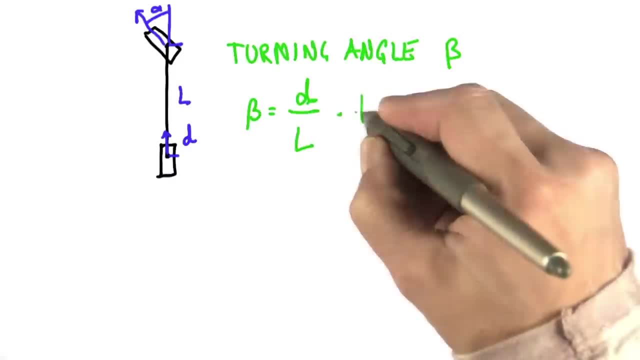 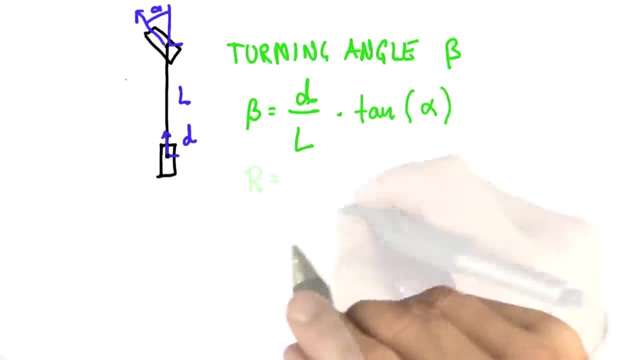 divided by the length of the vehicle times, the tangents of the steering angle, To now compute the changes of x, y and theta in the local coordinate system, we realize the turning radius r of this robot is simply the distance that we drive forward, divided by beta. 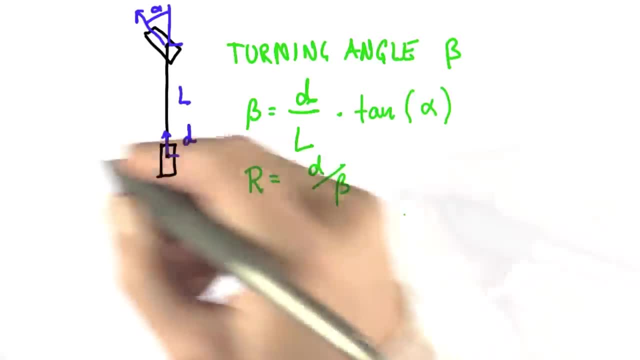 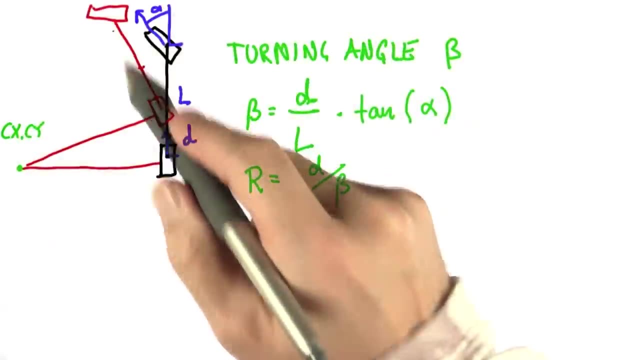 So it's relatively simple math, which I don't want to explain in detail. This means that the robot is turning around a point over here called Cx and Cy, and after the turn the vehicle is located somewhere over here In global coordinates. here's the way we describe this. 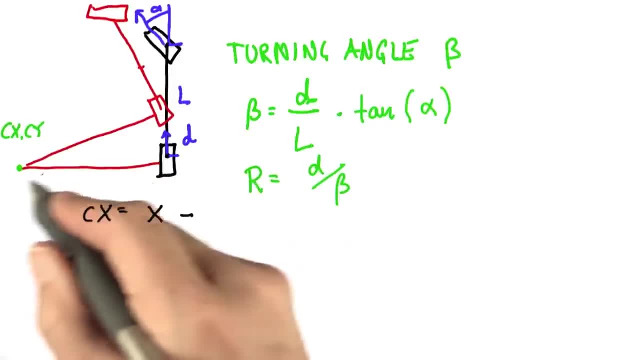 Cx is the x coordinate of the robot, x minus. now we go to the left. the sign of the robot: orientation before motion times. radius r. Similarly, Cy is this: Cy, is this expression over here, y plus cosine of the orientation times r. 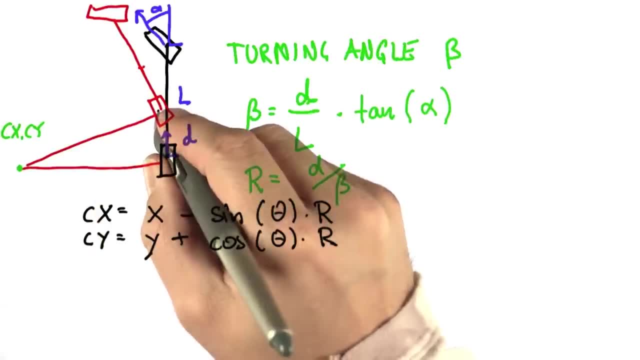 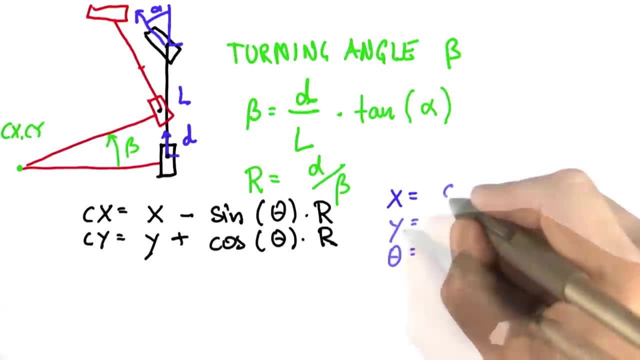 Then after motion we can go back from Cx to Cy, to a new state over here, simply by adding in the turning radius beta. That is our new x is Cx plus sine of theta plus beta times radius- Notice how this parallels this guy over here- except for two changes. 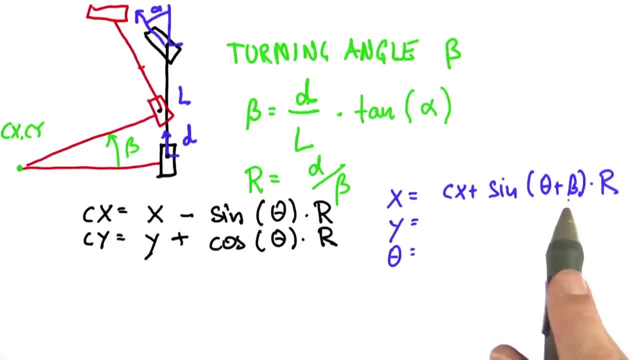 What we previously subtracted, we're now adding, and we're adding beta to the argument of the sign, Same with y, and the orientation is just increased by beta modulo 2 pi. Now this all works if the robot is actually turning. 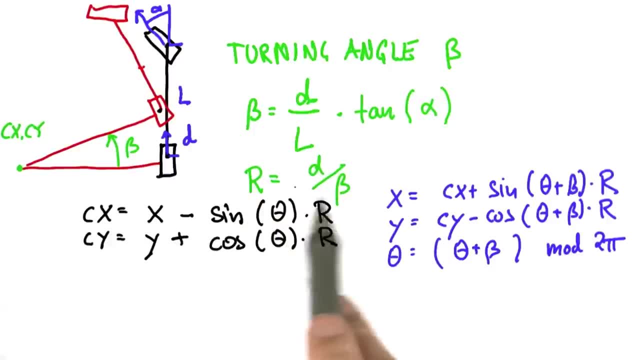 If the robot were to go straight then r would become infinity by this division over here. So for small betas you might call this smaller than 0.001.. We can approximate this all as straight motion. Our new x is the old x times our driven distance. 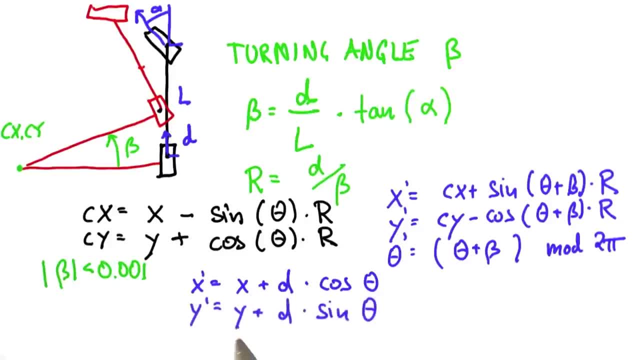 pointed in the cosine of the heading direction. Similarly, for y we go in sine of heading direction and the heading direction stays the same. You could add beta, which is basically 0, to be slightly more precise, or you could just use theta. 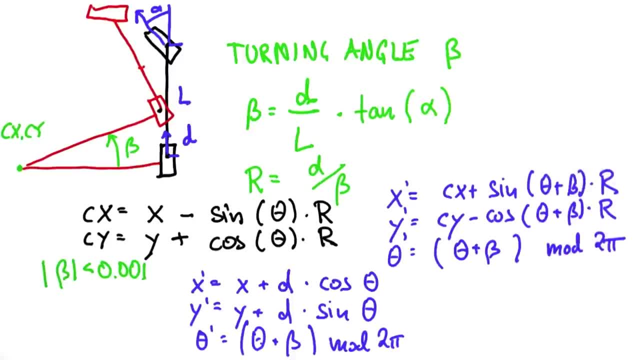 It doesn't really matter. In this programming assignment, I'd like you to implement this piece of math over here in our particle filter and to make sure we implemented it correctly. I will give you some example data that you can check. In our first part I prepared a lot of software for you. 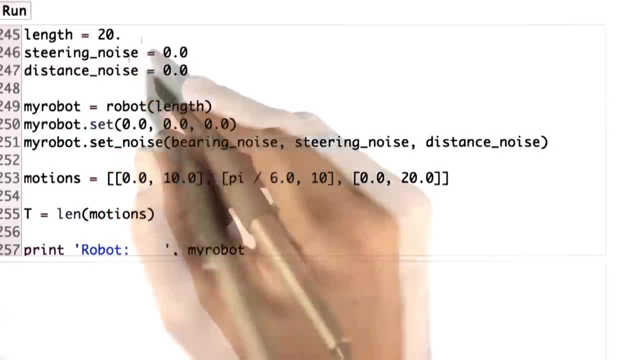 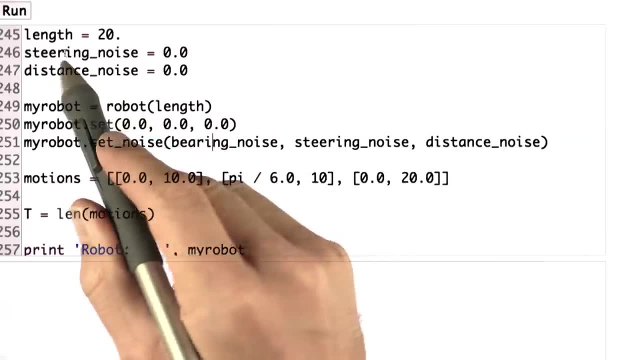 basically copying the old particle filter software over and removing the motion and the measurement model. for now, In this case, I just want you to practice the motion model. We assume a length of the robot of 20.. We initialize the robot with this length parameter. 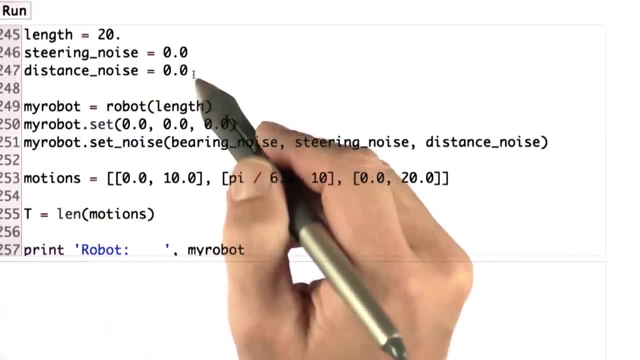 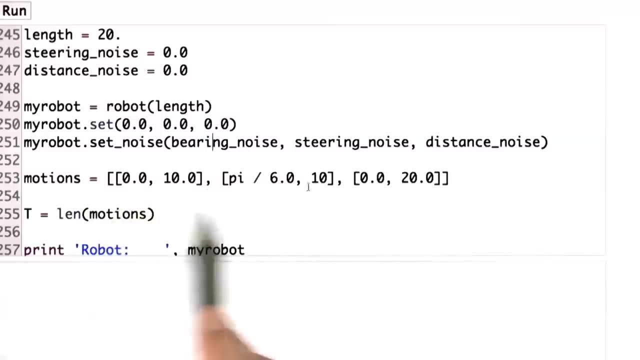 and for this first iteration we assume no steering noise and no distance noise. I set the robot to 0, 0, 0 in the beginning and then I cache away a number of motions and the way to read those is: this robot is moving by 10 in total. 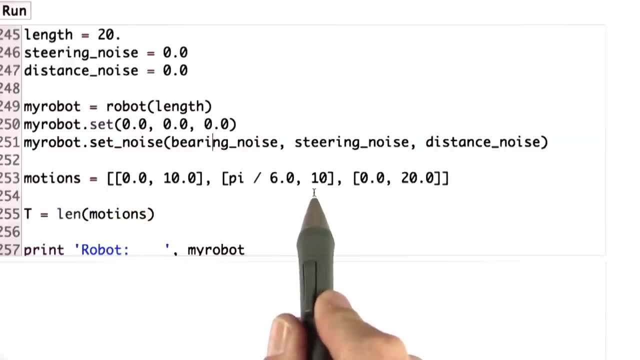 with a steering angle of 0.. Then it moves another 10 with a steering angle of pi divided by 6, and then it moves 20, again with a steering angle of 0.. A pi over 6 is a left steering, so the robot should change its coordinates in the beginning just in the x direction. 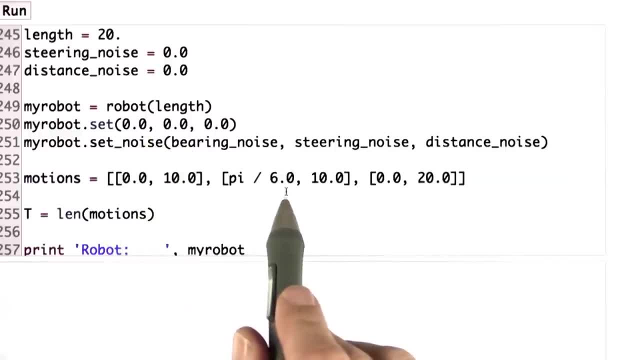 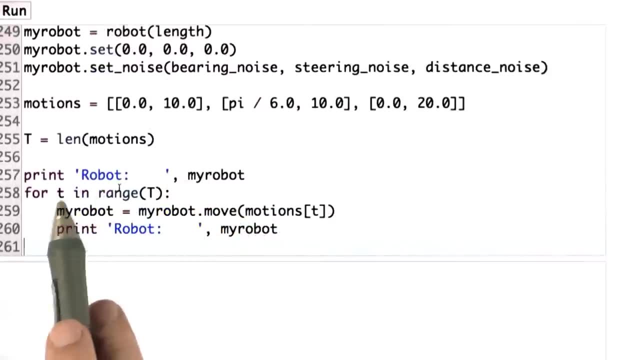 because it's facing an x direction over here. Then turn left a little bit, go forward and go straight again. Scrolling down a little bit, I also give you the code to run the robot. We've created it over here. We print the initial coordinate. 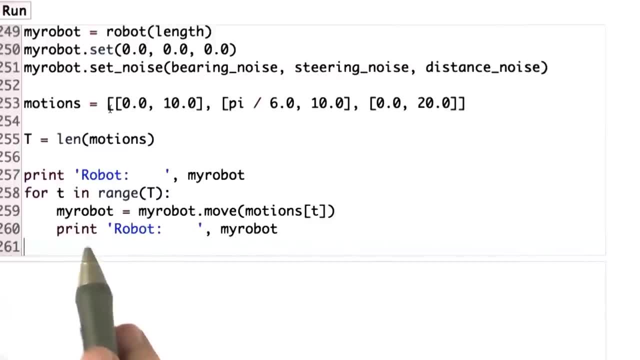 and then, for each of the motions in this list over here, we apply the myrobot equals myrobot move command and we print out the successor command. If you get this right, this is the numbers I would like to see. Initially, the robot position is 0, 0, 0. 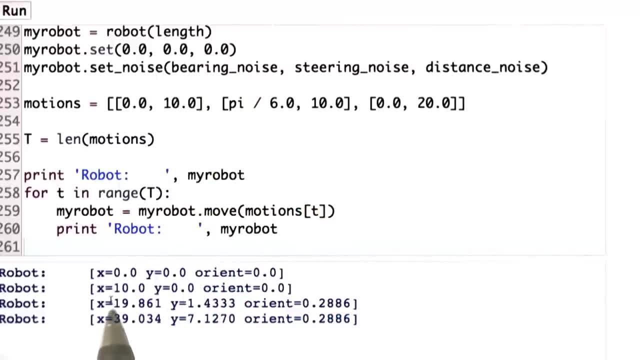 That's just the one over here. It's our first print command. It then moves forward in x direction by 10.. Orientation stays 0, so does y, because there's no steering. Now we steer, This affects x. It doesn't quite move 10.. 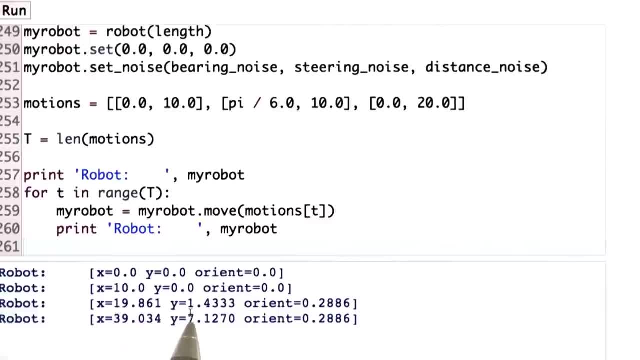 It only moves 9.86.. In y direction it moves 1.433, and its new orientation is 0.2886.. Then we move straight again, and now the x coordinate becomes 0.3903.. y coordinate becomes 7.12,, orientation 0.28.. 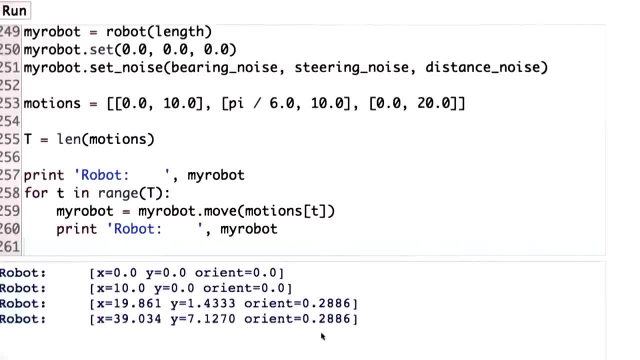 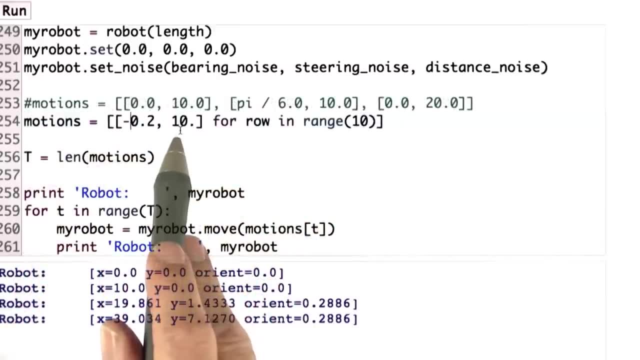 Your code should output exactly the same values, Of course, over here. Just to give you a second test. this is a sequence of 10 motions where the robot always moves 10 forward and always turns right by an angle of 0.2 in radians. 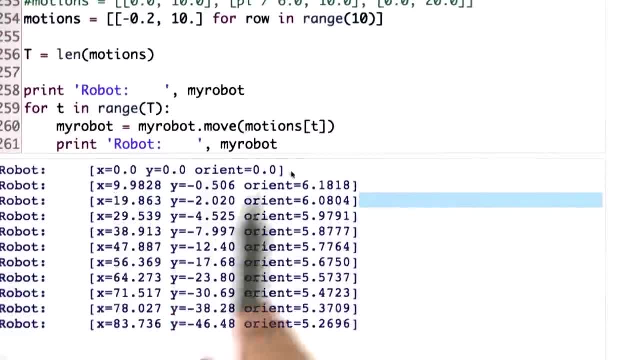 We look at the outputs, then we get the following array. You can see that the orientation starting at 0,, which is the same as 2 pi, decreases all the way to 5.26.. You can also see the robot starts running in a circle. 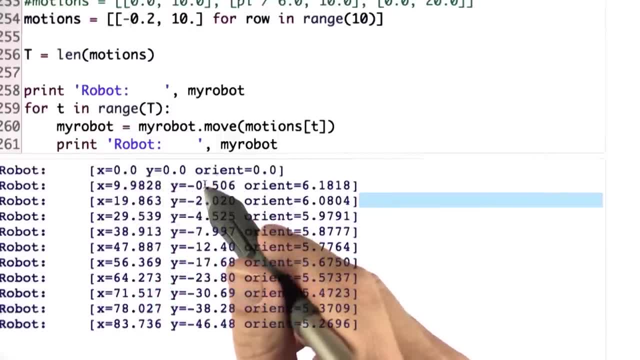 whereas initially we add almost 10 to the x direction, almost nothing to the y direction, As we come down here we subtract quite a bit in y direction, because now the robot is going on a circle. You should look at these numbers over here. 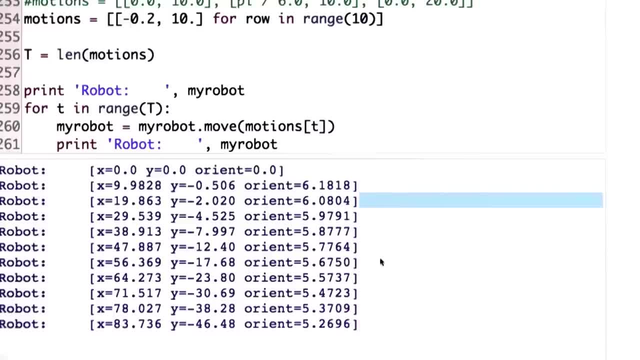 and see if your code matches these exact numbers that my code outputs. 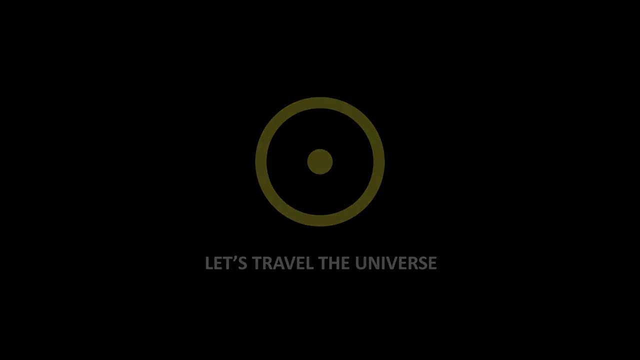 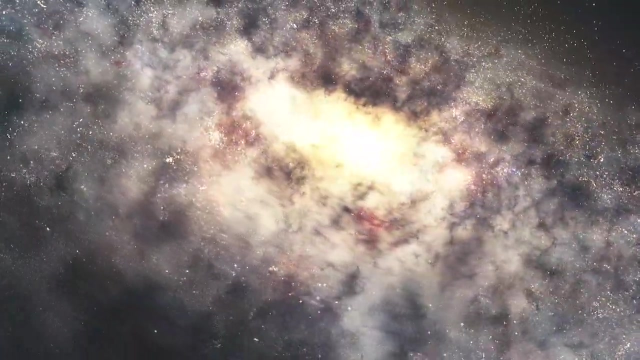 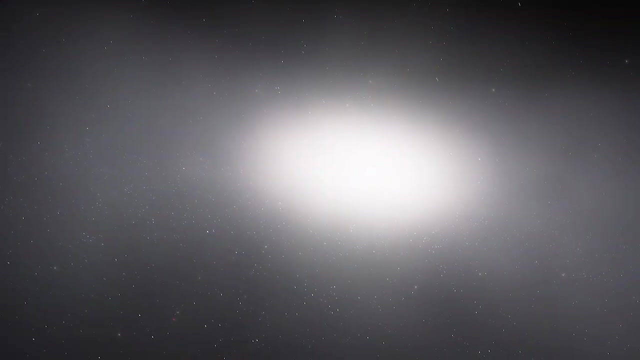 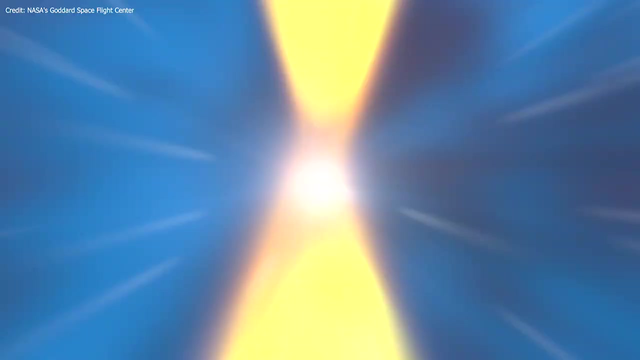 Most of the galaxies we observe are considered normal. We inhabit a normal galaxy called the Milky Way. When you observe a normal galaxy, most of the light comes from the star's invisible wavelengths and is evenly distributed throughout the galaxy. But if you look at some galaxies, you will see intense light coming from their nuclei. 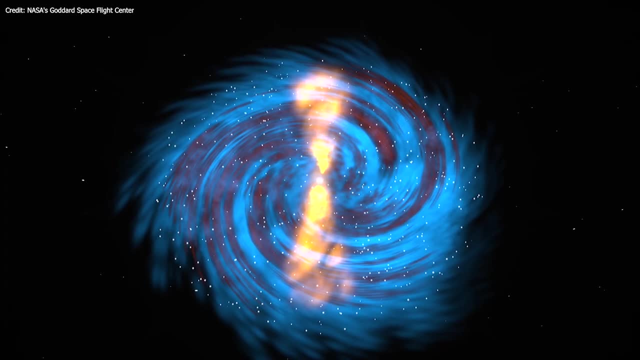 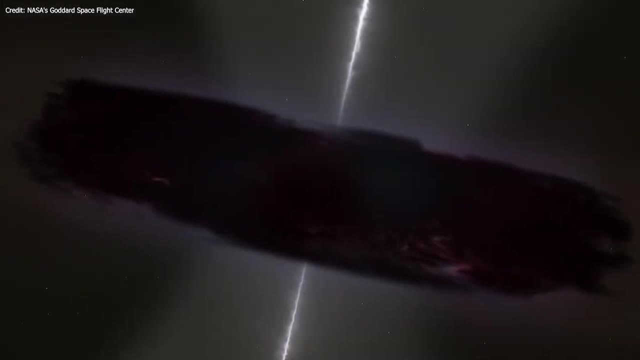 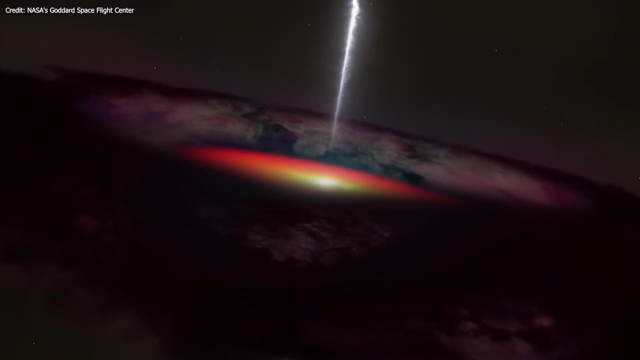 These are active galaxies. An active galaxy emits up to thousands of times more energy than a normal galaxy, But most of this energy is released not in visible light but other wavelengths, from radio waves to gamma rays. These types of galaxies represent a very different type of energy. 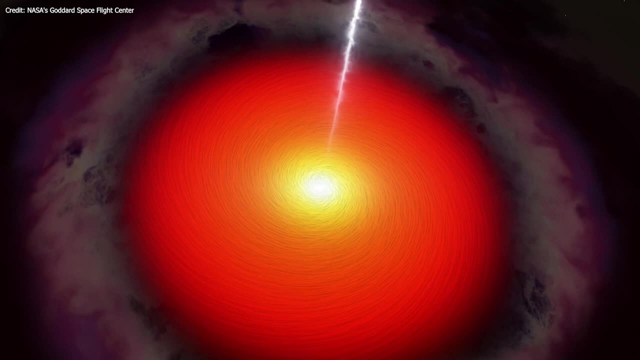 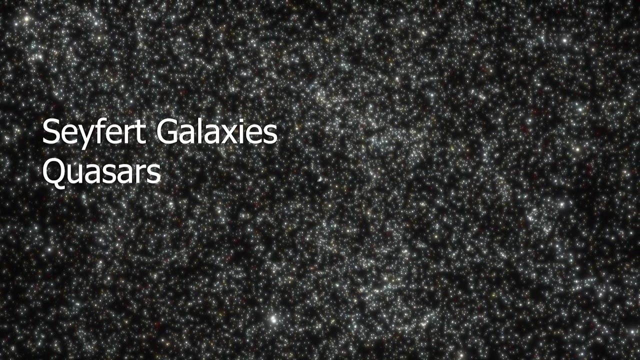 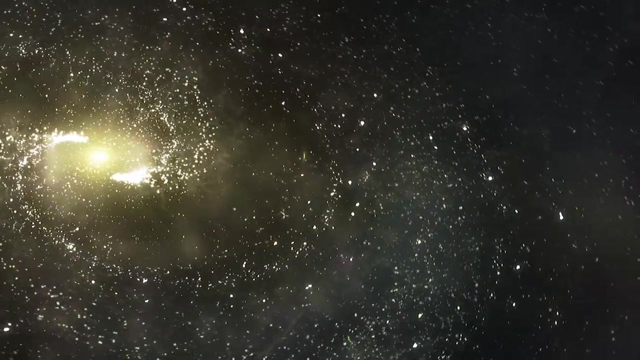 They are a very small percentage of all galaxies we've detected. There are four types of active galaxies, including ciphered galaxies, quasars, blazars and radio galaxies. Ciphered galaxies are active spiral galaxies. Its nucleus has bright emission lines, including visible wavelengths.